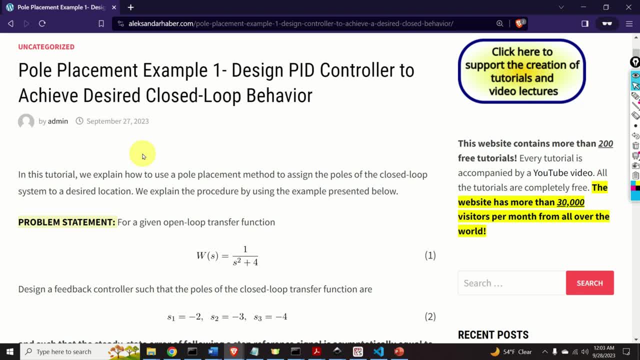 Hello everyone and welcome to control engineering tutorials. In this tutorial, we will solve one very important problem that every control or signal processing engineer need to know how to solve. Namely, in this tutorial, we will learn how to use the pole placement method to select control algorithm parameters. 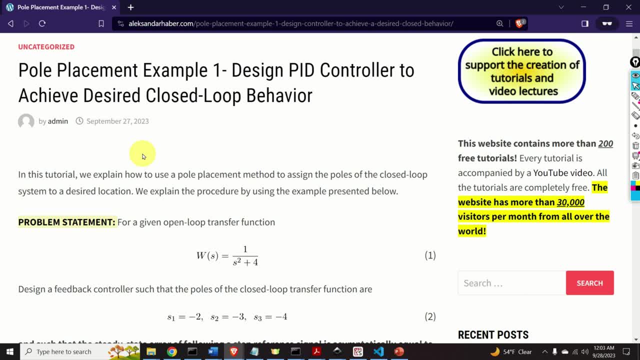 such that the poles of the closed loop system are placed at the desired locations and such that the desired closed loop behavior is achieved. More precisely on the basis of the desired locations of the closed loop poles, we will determine the parameters of the proportional integral derivative. 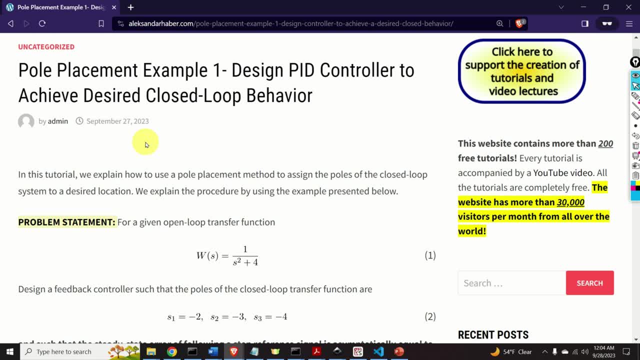 or PID control algorithm. We will also see that the control algorithm will introduce zeros in the closed loop transfer function. that will slightly degrade the desired closed loop response. But before I start with explaining the control algorithm, I would like to start by explaining the control algorithm. 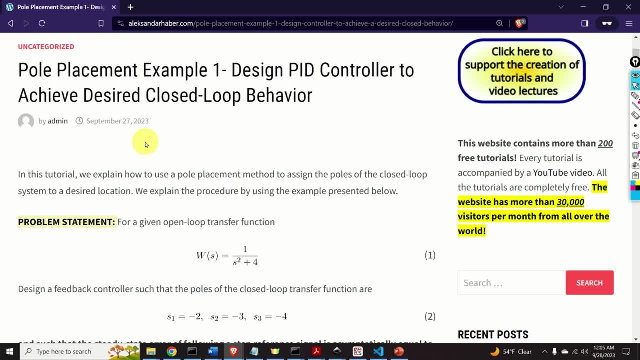 I would like to mention the following. It took me a significant amount of time, energy and planning to create this completely free video tutorial, as well as more than 350 free video tutorials that you can find on my youtube channel, and consequently, I kindly ask you: 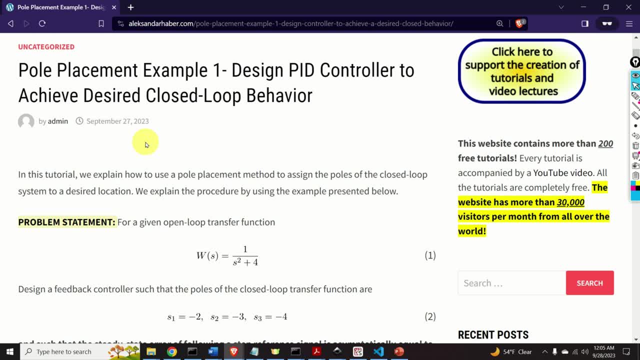 to press the like and subscribe buttons. Thanks a lot. Also, if you have any question or a comment about the material presented in this video tutorial, please feel free to leave your comment below. If you have any question or a comment, or a question in the comment section below this video tutorial. 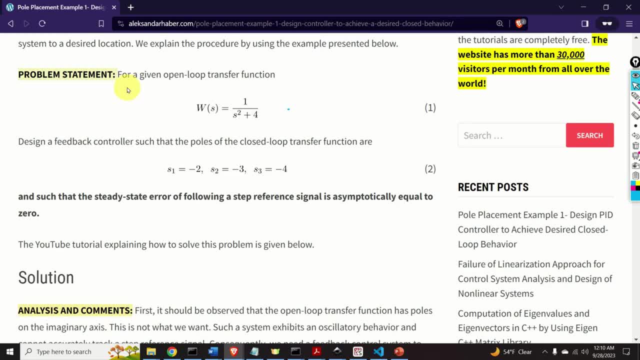 Thanks a lot. Here is the problem statement. We are given an open loop transfer function, given by this equation, and we want to design a feedback control algorithm such that the poles of the closed loop transfer function are placed at these locations, at minus 2, minus 3 and minus 4.. 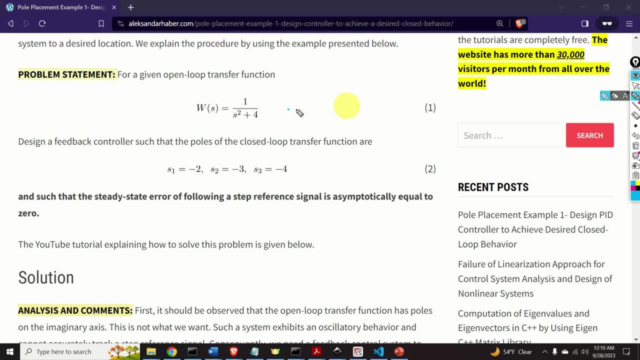 Here is what we should achieve. The poles of the open loop transfer function are on the imaginary axis, That is, one is at 2j and another one is at minus 2j, And we want to design a closed loop controller such that the poles 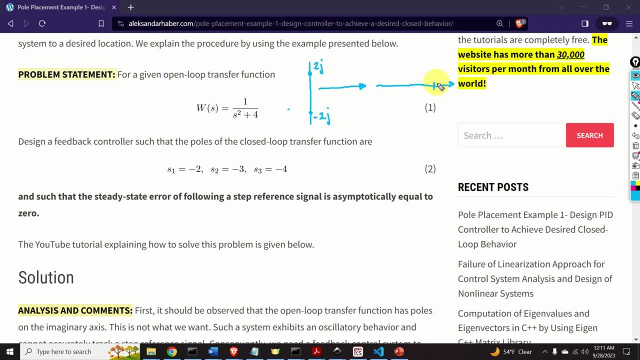 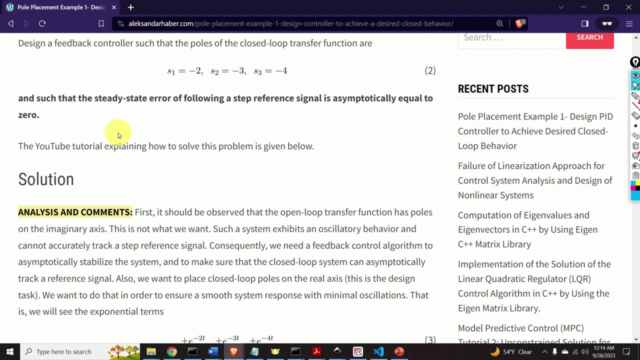 of the closed loop transfer function are placed at minus 2, minus 3 and minus 4.. Also a very important design requirement is that the steady state error of following a step reference signal is asymptotically equal to zero. Let's solve this problem. 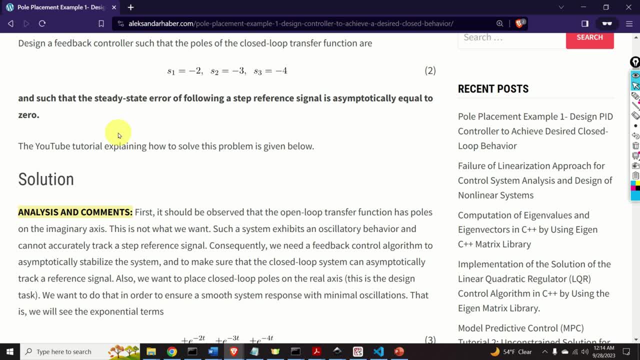 The first step is to analyze the problem and to explain a few important things. As I mentioned previously, it should be observed that the open loop transfer function is located at the bottom. function has poles on the imaginary axis. This is not what we want. Such a system exhibits an 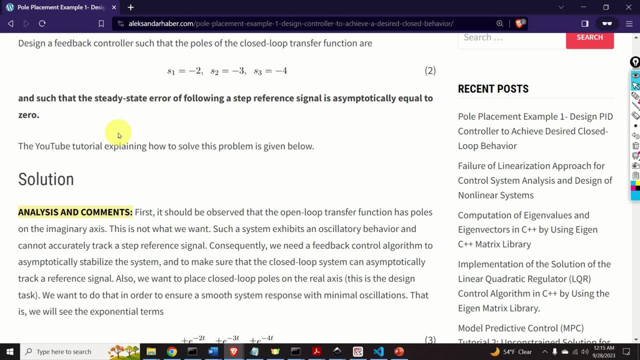 oscillatory behavior and cannot accurately track a step reference signal. Consequently, we need a feedback control algorithm to asymptotically stabilize this system and to make sure that the closed-loop system can asymptotically track a reference signal. Also, we want to place 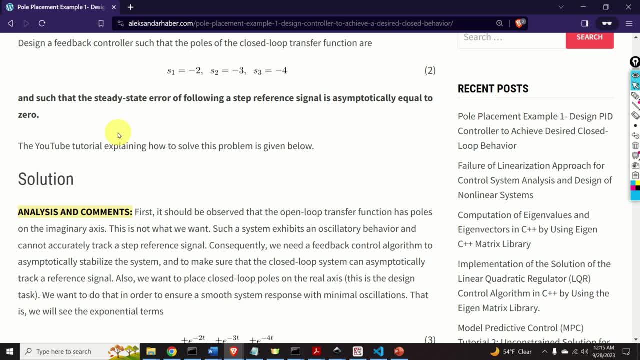 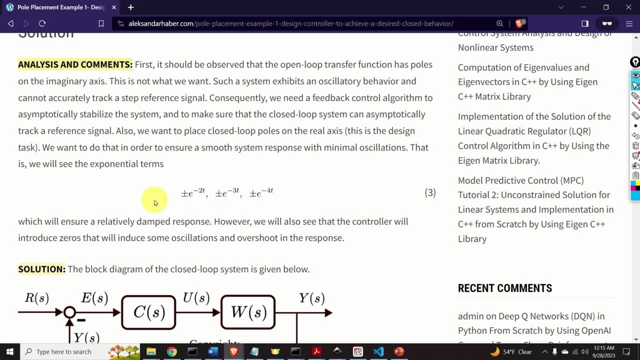 closed-loop poles on the real axis. We want to place the closed-loop poles on the real axis mainly because we want to ensure a smooth system response with minimal oscillations, That is. we will see that these exponential terms will appear in our step response. However, we will also see 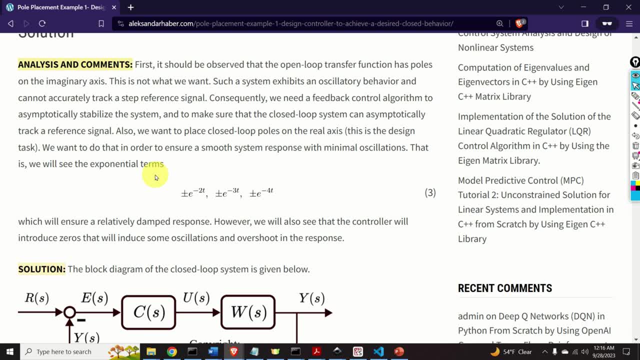 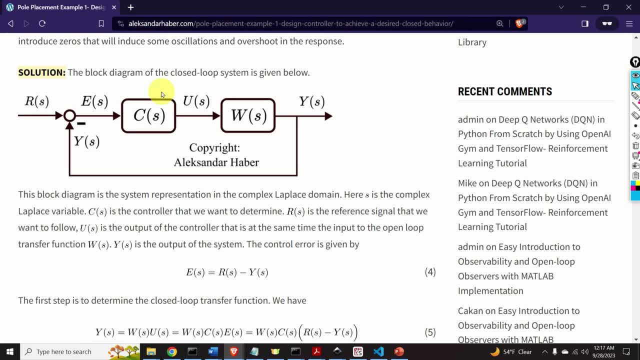 that the controller will induce zeros. that will induce some oscillations and overshoot in the response. Now we understand the requirements and we understand why the problem is formulated like this. The next step is to solve the problem. The first step in our solution is to construct the block. 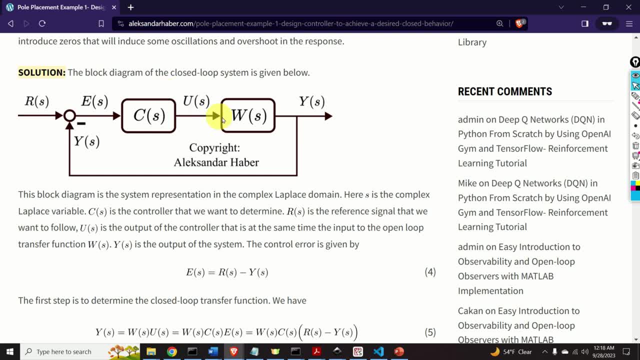 diagram of the system. Here is the block diagram. W is our open-loop transfer function. C is our controller. S is the Laplace complex variable. E is the open-loop transfer function. Error in the Laplace domain and error is the difference between the reference signal. 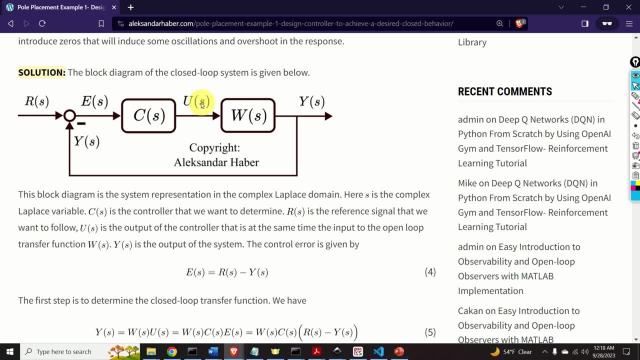 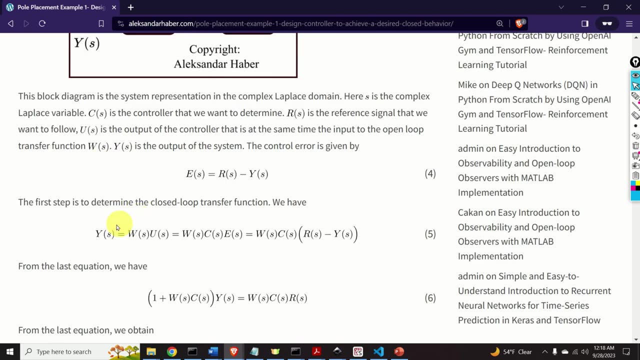 and the output of the system. U of s is the output of the controller that is, at the same time, the input to our open-loop transfer function, And here is the feedback. Next, we need to determine the closed-loop transfer function, The closed-loop transfer. 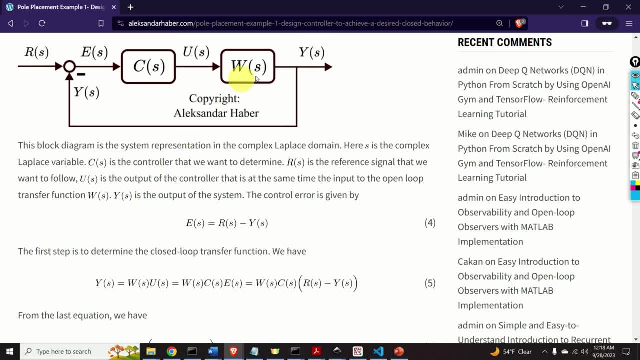 function is derived from this equation. What do we do over here? We simply write the output as a product of our W and U and we go one step back. We know that U is actually E times C and we substitute these equations in this equation and finally, we substitute the expression. 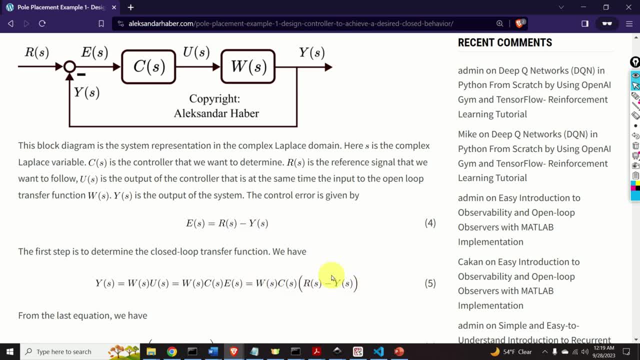 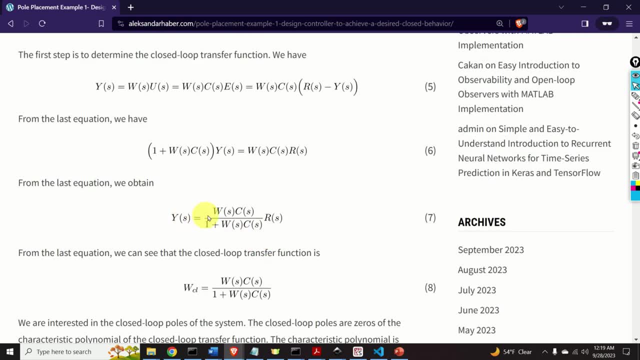 for the error given over here, and we obtain this equation From this equation. we obtain this equation and from this equation we obtain this very important equation. This is the input-output representation of our closed-loop transfer function. This is the closed-loop transfer function. R is a reference signal. This signal is the desired behavior of our 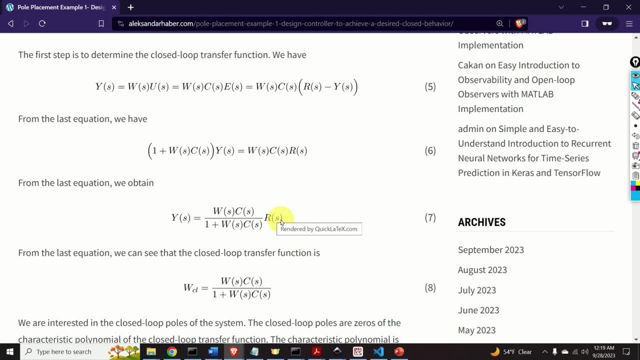 output and this signal is specified by the user. For example, it can be a step signal, it can be a ramp signal, it can be a sinusoidal signal or it can be a combination of these elementary signals. We filter this input signal through our transfer function to obtain the 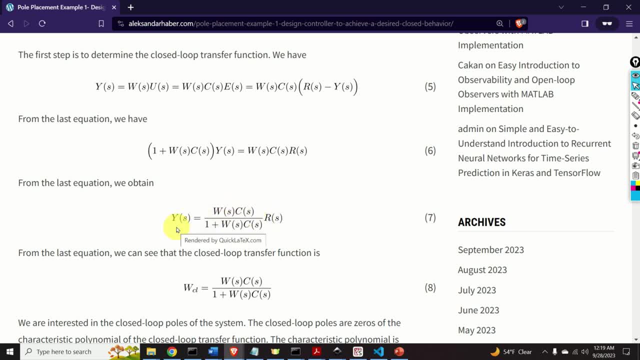 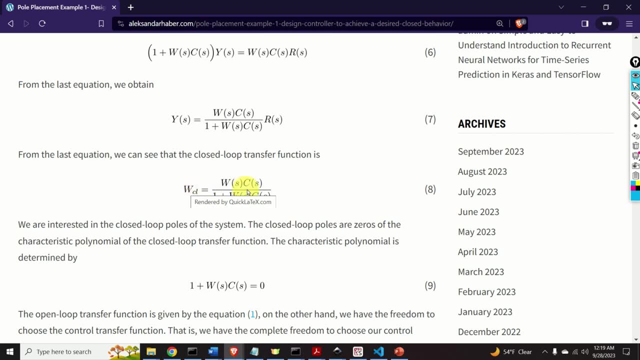 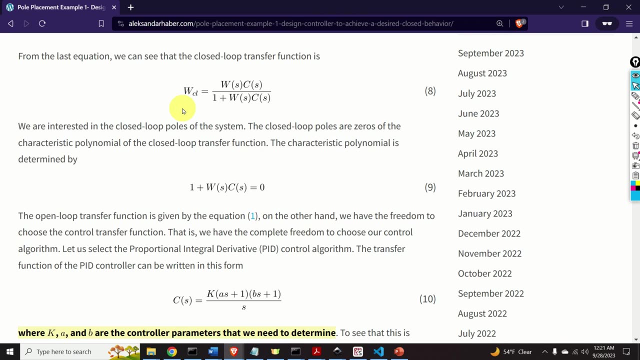 output of the system. This transfer function is, for example, a signal from our current called the closed loop transfer function, and it's given by this equation. Another very important concept that we need to define is the concept of the closed loop characteristic polynomial. 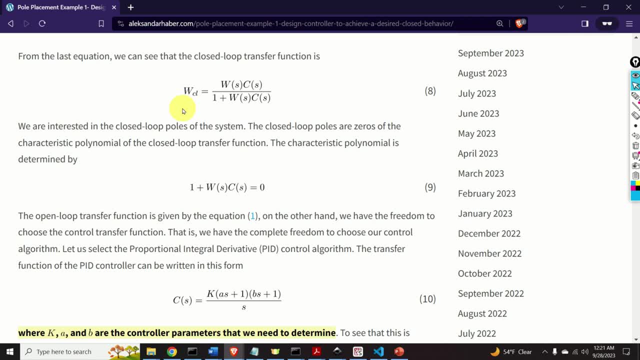 The closed loop characteristic polynomial is obtained by setting this expression in the denominator of our transfer function to zero and consequently we obtain this equation. From this equation, we will obtain the closed loop characteristic polynomial. Let's analyze this equation. W of s is given. 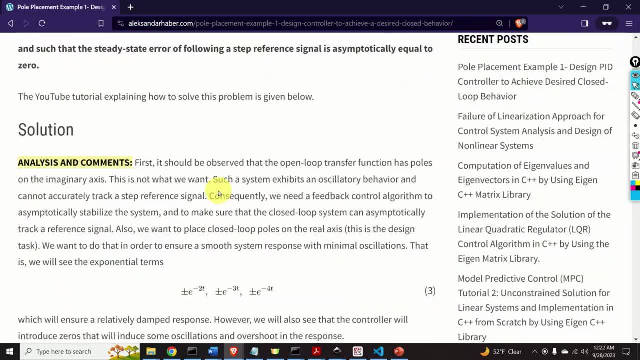 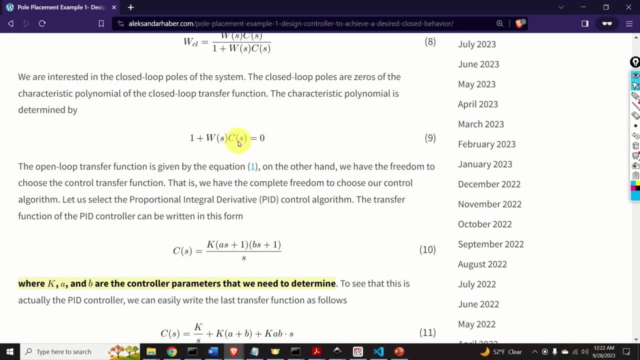 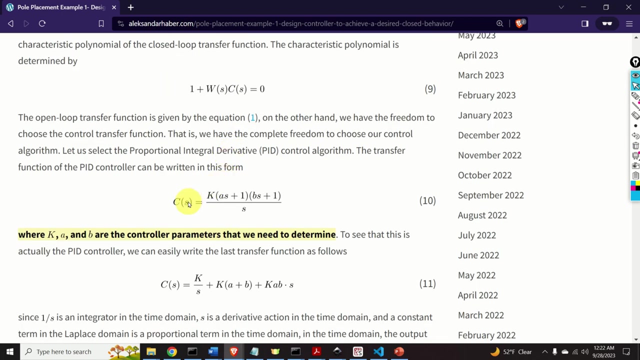 This is our open loop transfer function. given by this equation, However, we have a complete freedom to choose our controller. In this video tutorial, I will select the proportional integral derivative, or PID control algorithm. The transfer function of the PID control algorithm can be written like this: 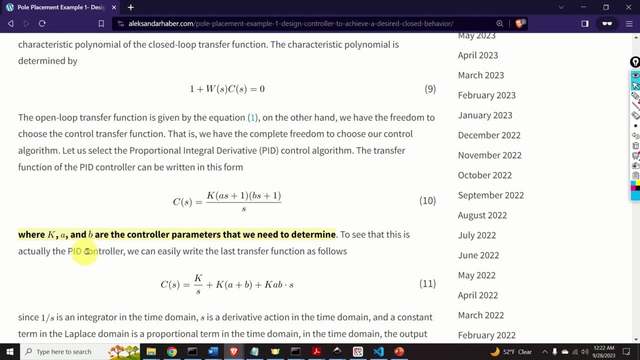 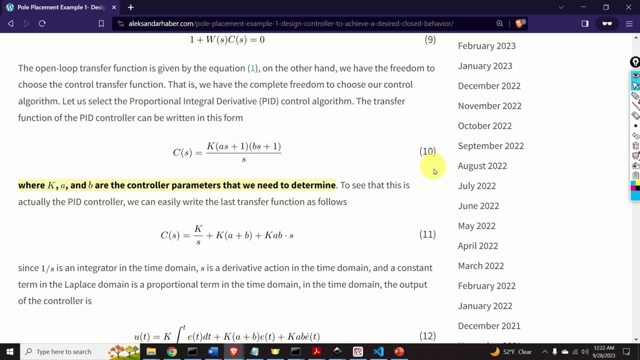 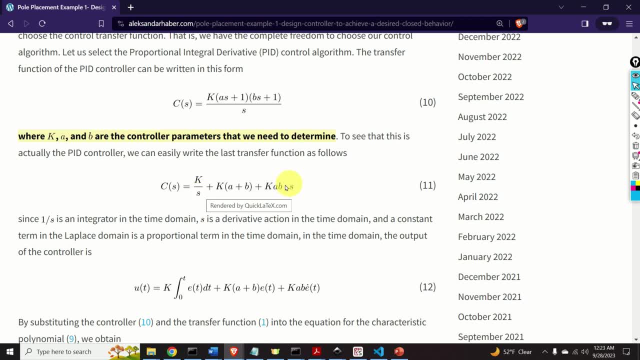 Since 1 over s is an integrator in time domain. Since 1 over s is an integrator in time domain, S is the derivative in the time domain and a constant term in Laplace domain is a proportional term in the time domain. 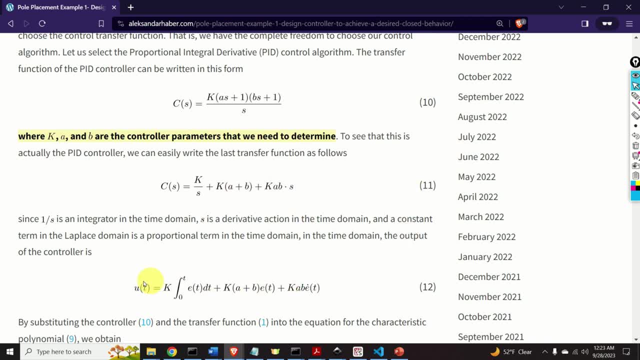 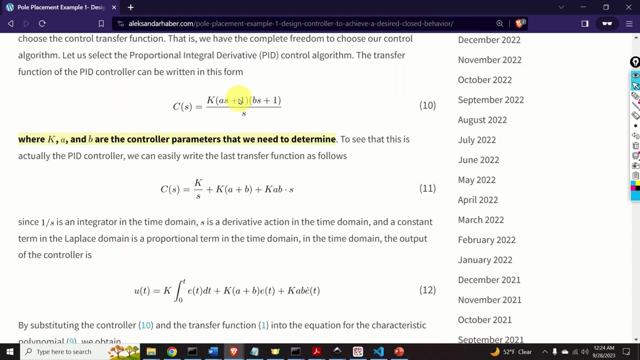 In the time domain. this equation has this form And we can clearly see an integral term corresponding to this part, Proportional term over here corresponding to this part And derivative term corresponding to this part, transfer function and our controller in this equation. As the result, we obtain this equation. 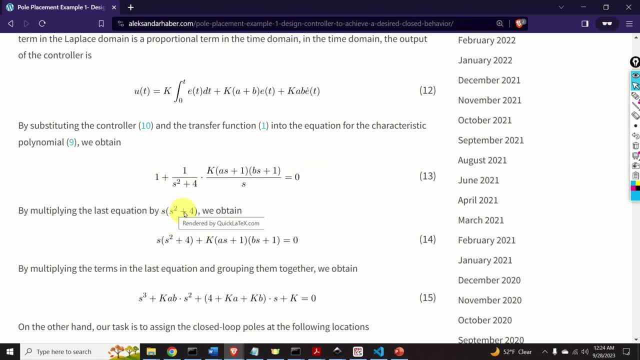 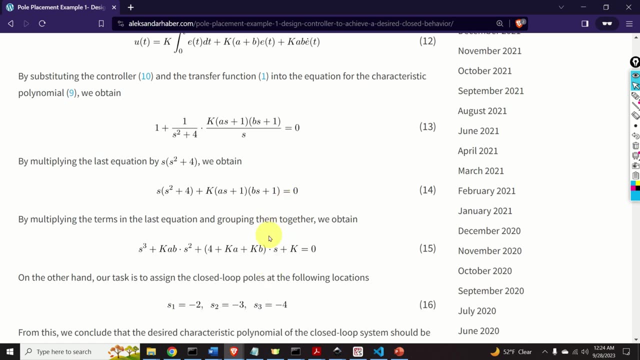 By multiplying this equation by s multiplying s squared plus 4,, we obtain this equation, And by multiplying the terms in this equation and grouping them together, we obtain this equation. On the other hand, our task is to assign the closed loop poles at the following: 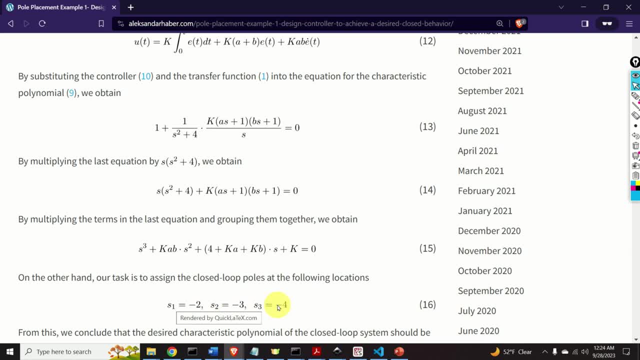 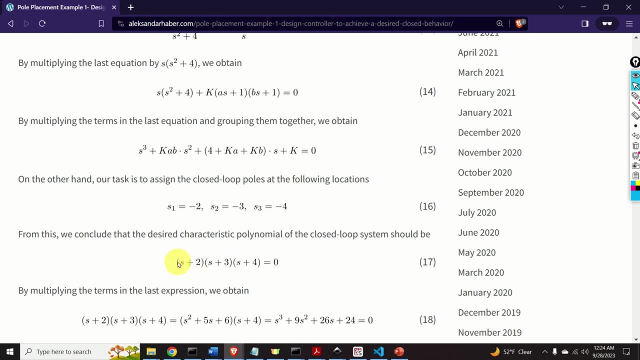 locations minus 2,, minus 3, and minus 4.. From this we conclude that the desired characteristic polynomial of the closed loop system should look like this: How do we know that? Well, if we substitute s1 over here, we obtain 0. If we obtain, if we substitute minus 3 over. 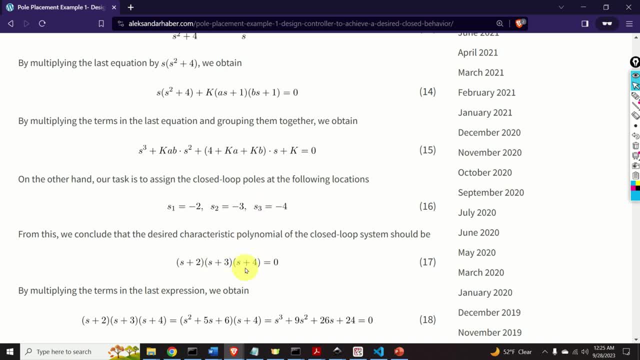 here we obtain 0.. If we substitute minus 4, we obtain 0. That is, this is our desired closed loop characteristic polynomial Subtitles by the Amaraorg community. by multiplying the terms in this expression, we obtain this equation And finally we obtain. 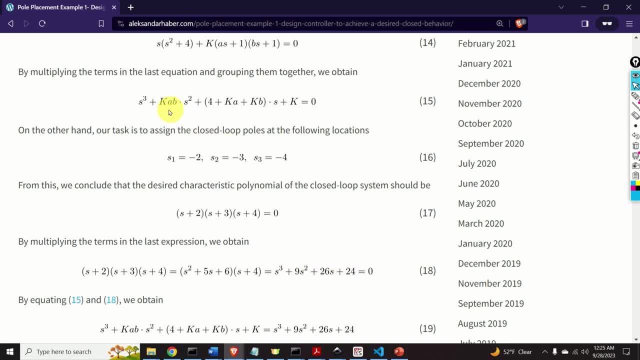 this polynomial. Now we want to select k, a and b, such that this parametrized characteristic polynomial is equal to desired characteristic polynomial. And what do we do? We simply say: this equation should be equal to this equation And consequently, we obtain this equation. 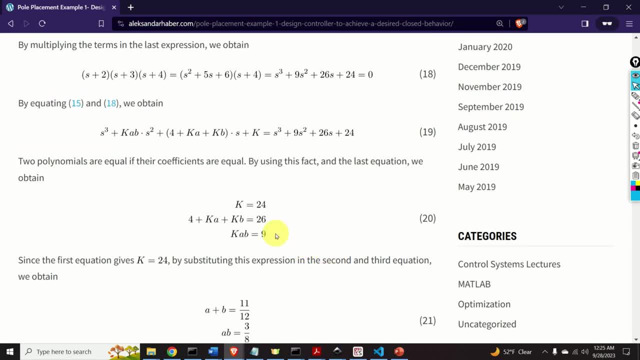 We know that two polynomials are equal if their coefficients are equal. By using these factors and this expression, we obtain- Let's see: k is obviously equal to 24.. Perfect, This term: 4 plus k a plus k b should be equal to 26.. Here's our second equation, And 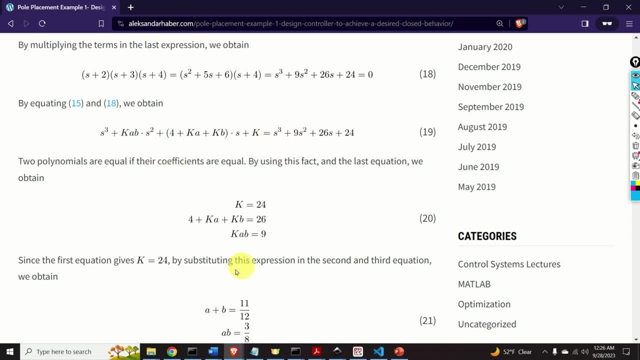 where's our third equation? Here it is: k a- b should be equal to 9.. Here it is: Subtitles by the Amaraorg community Of this term: four plus k a plus k b should be equal to 26.. And where's our third equation? Here it is: k a, b should be equal to 9.. Here it is. From the first equation we immediately obtain that item k, a and b should be equal to 9, here it is, and it is key scientists. 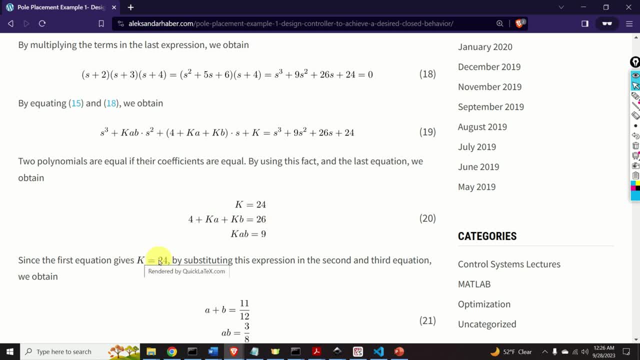 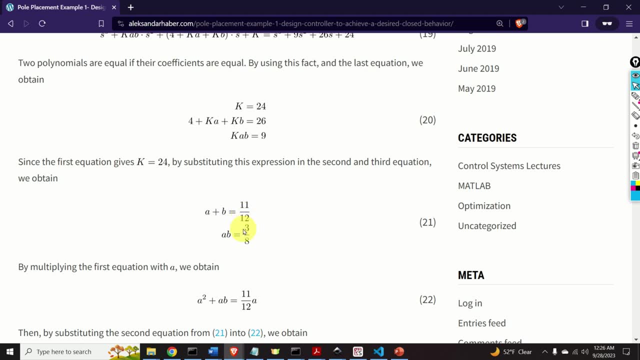 The first equation, we immediately obtain that k is 24.. And by substituting, k is equal to 24. in these two equations we obtain the set of equations in the equation 21.. This is a system of two equations in two unknowns. The unknowns are a and b. 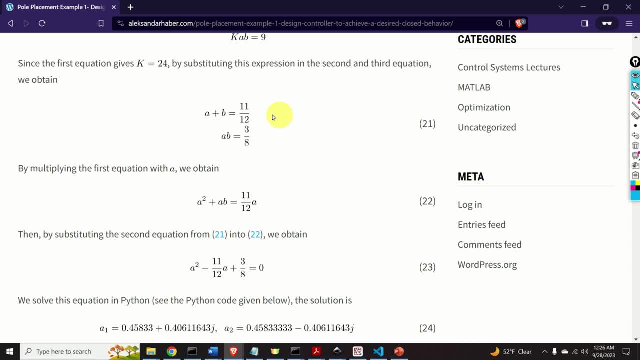 And let's solve this system. Let us first multiply the first equation from left with the a And as the result we obtain this equation. And over here we can see this term a, b. So substitute a, b in this equation and finally you will obtain this equation. 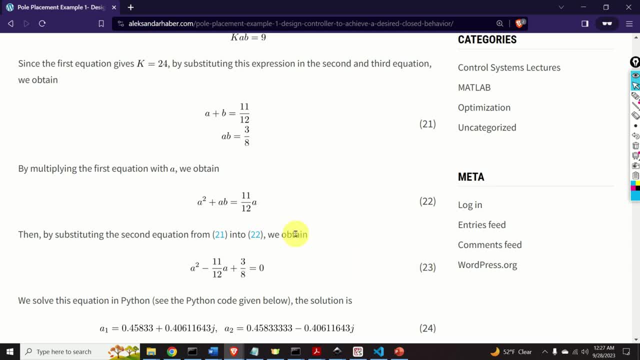 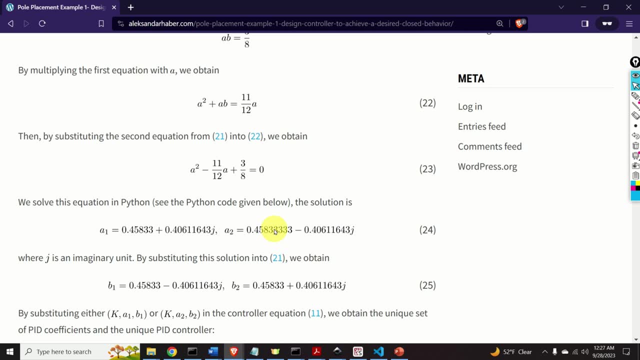 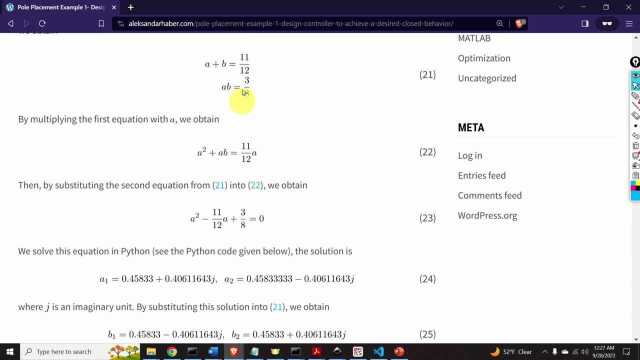 I will solve this equation in Python and later on I will show you the code. The solution is given over here. Here it is: We have a1 and a2.. Corresponding to a1, we also have b1.. b1 is obtained from this equation by simply dividing this expression by a2.. 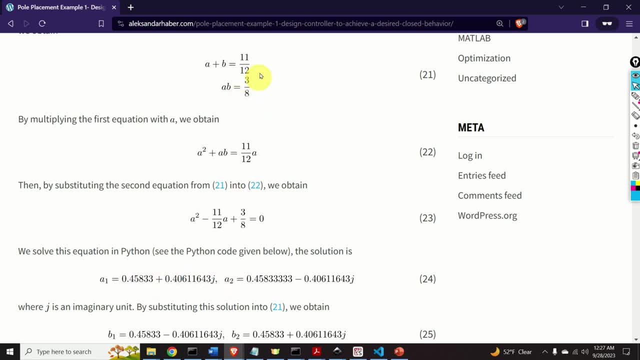 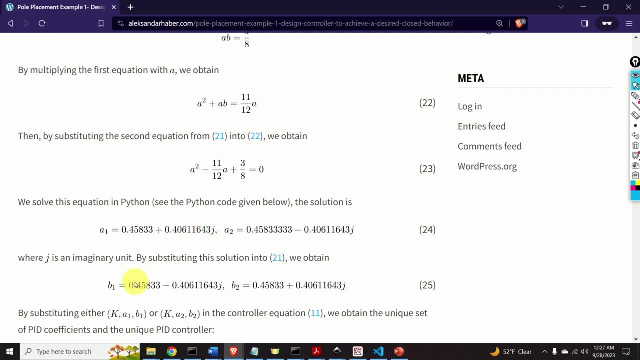 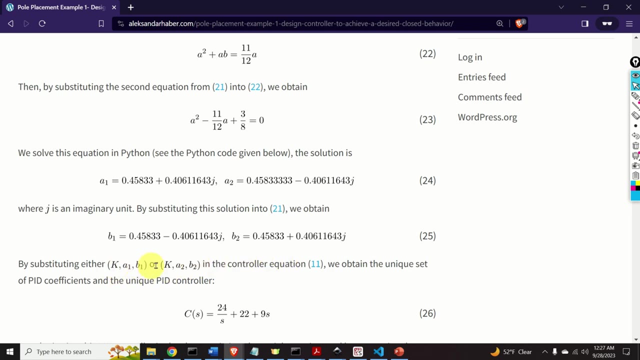 And watch out. a is a complex number, and be careful when dividing the complex numbers. I do that in Python And as the result, we obtain b1 and b2.. So we have two sets of control parameters. We have this set and we have this set. 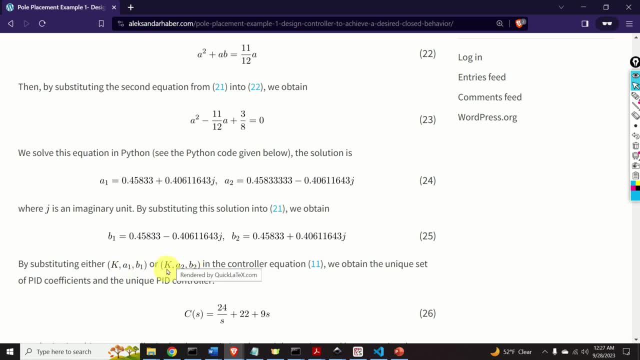 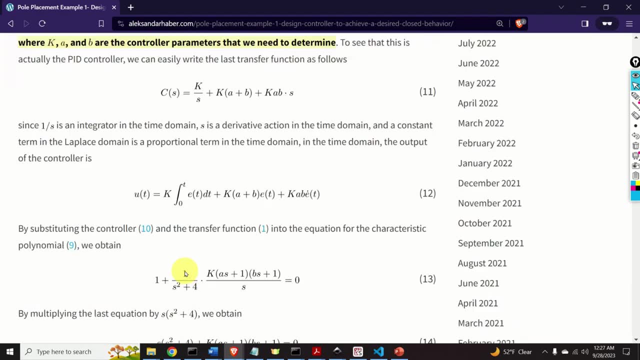 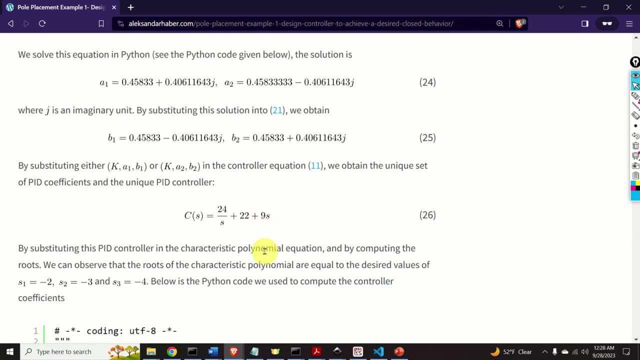 If we substitute these control parameters. you can choose any set, for example, either this one or this one, And you substitute them In our PHP. Let's see: We will obtain the PID controller equation. either in this equation or in this equation, You will finally obtain the PID controller. 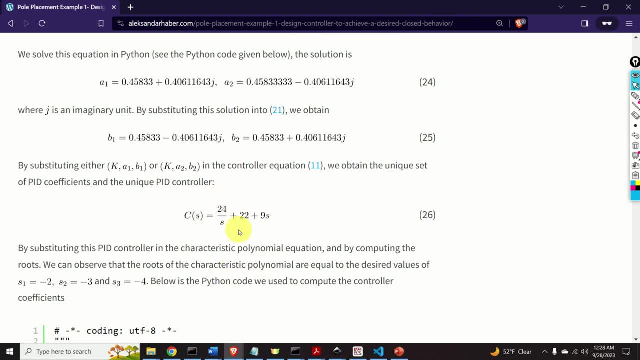 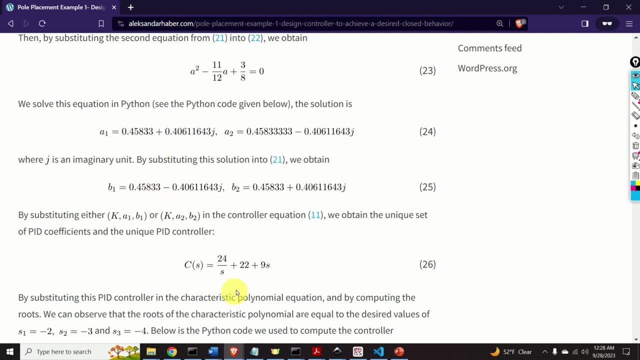 Here it is Now. here you need to observe the following: The parameters a1 and b1 are complex. However, since we have multiplication of complex parameters, we will obtain controller that doesn't depend on complex parameters And, consequently, this controller can be implemented in your digital computer. 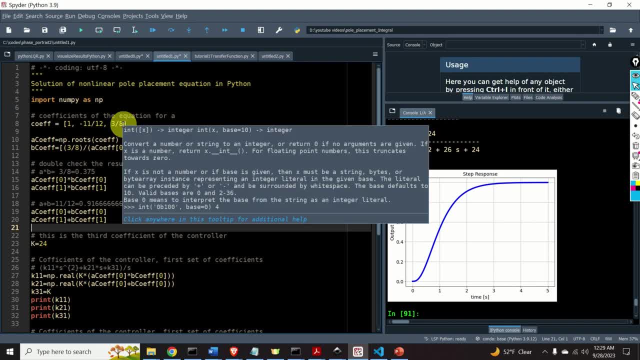 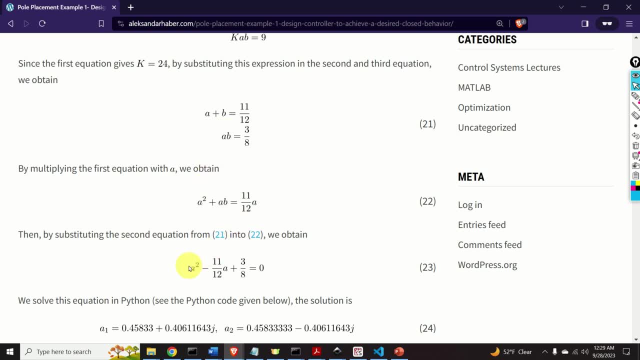 Perfect. Here is the Python code for computing the parameters a and b. First we want to solve this equation Over here, Or better to say this equation. We can do it easily in Python By first observing that this is a polynomial in a. 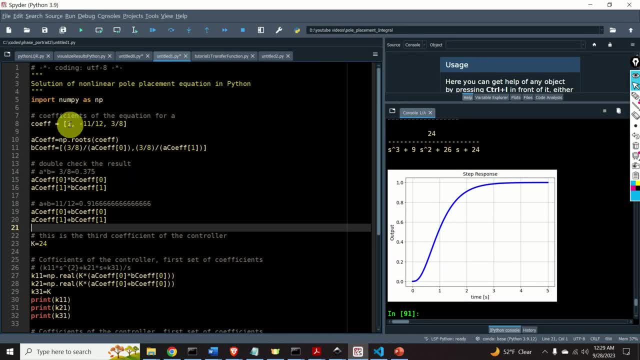 And we specify a list with the coefficients of this polynomial. We have b1.. b2.. b3., b4., b5., b6., b7., b8., b9., b10., b11., b12., b12. 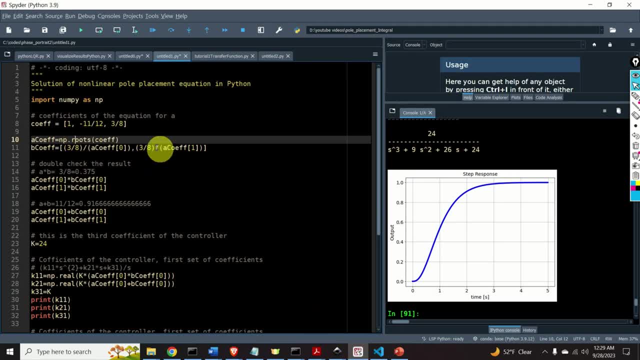 b13., b14., b15., b16., b17., b18., b19., b20., b21., b22., b23., b24.. b25., b26., b27., b28., b29.. b30., b31., b32., b33., b34., b35., b36., b37., b38., b39., b40., b41., b42., b43., b44., b45., b46.. 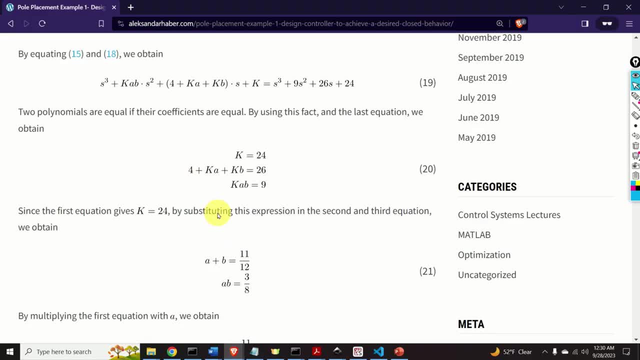 b47., b48., b49., b50., b51., b52., b53., b54., b55., b56., b57., b58., b59., b59., b30., b31., b32. b33., b34., b35., b36., b36., b37., b38., b39., b40., b41., b42., b43., b44., b45., b46., b46., b47.. b48., b49., b50., b52., b53., b54., b55., b56., b56., b57., b58., b59., b59., b59., b60., b60., b61. b62., b62., b63., b64., b65., b67., b68., b68., b69., b70., b71., b72., b72., b73., b74., b74., b75. 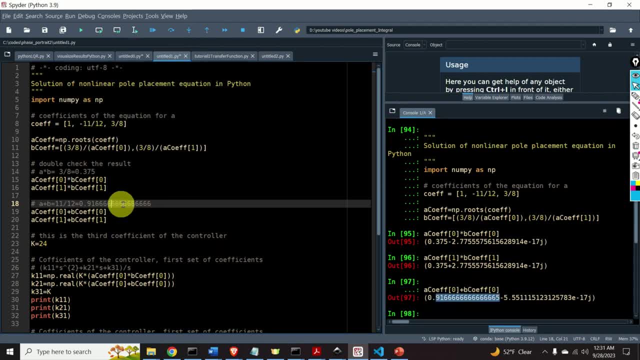 b76.. b78.. b79.. b20.. x dados bрод. b21.. b22.. b26.. b27. b28.. 0.966666.. b29. b20.. 0.9x66666.. 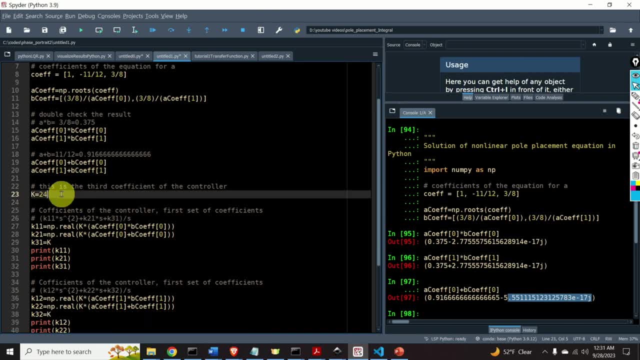 0.9x66666.. 0.9x66666.. 0.9x66666,, 0.9x66666, And we'll obtain exactly 0.9966666, And over here, of course, we have an imaginary part that's equal to zero. 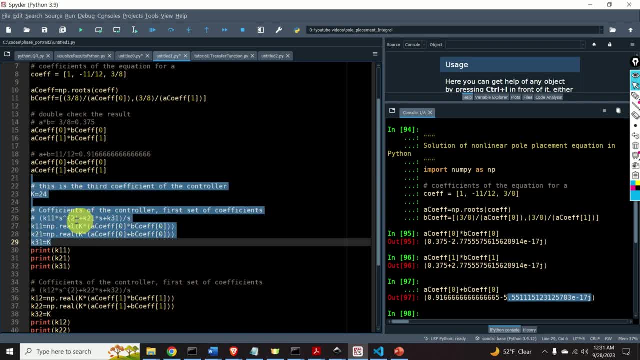 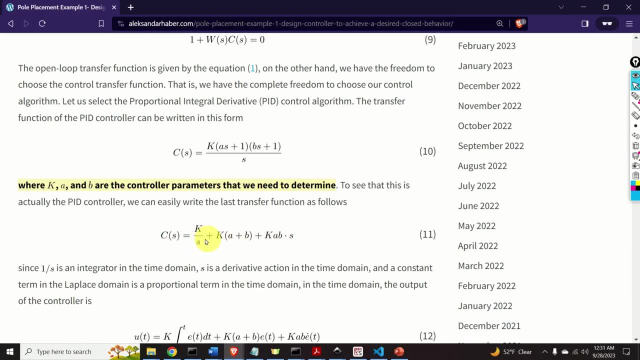 Next, let's compute the control algorithm parameters. We said K is equal to 24 and we simply compute the constants of the PAD controller. that is, we use this equation to compute the constant P8.. 8, 00.. of the integral action constant of the proportional action and the constant of. 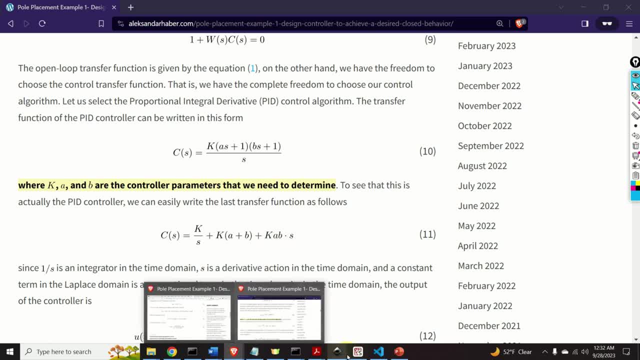 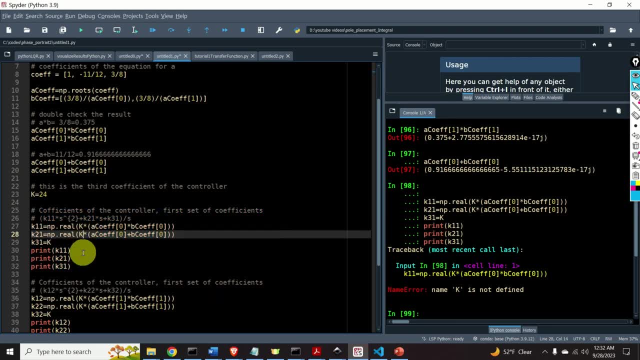 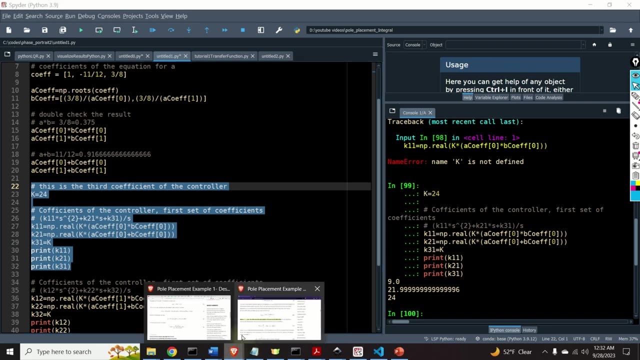 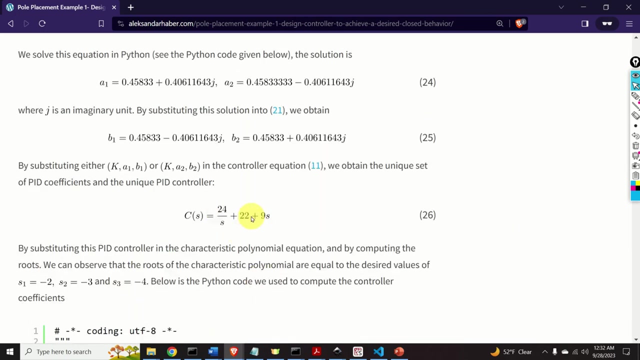 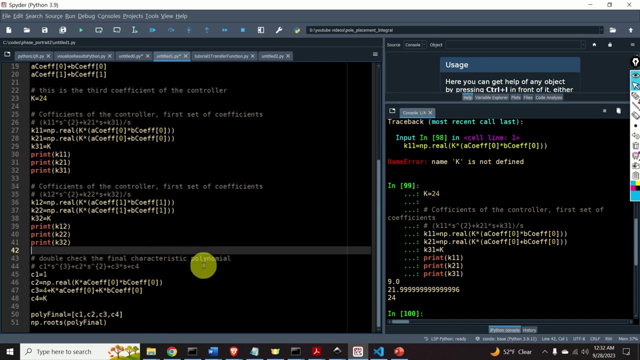 the derivative action. And here's how we do it in Python. Here the constant. We just need to select this part and here they are: 9,, 22 and 24.. Going back to the post, here they are 9,, 22 and 24.. Perfect, Let's continue. Let us double check the. 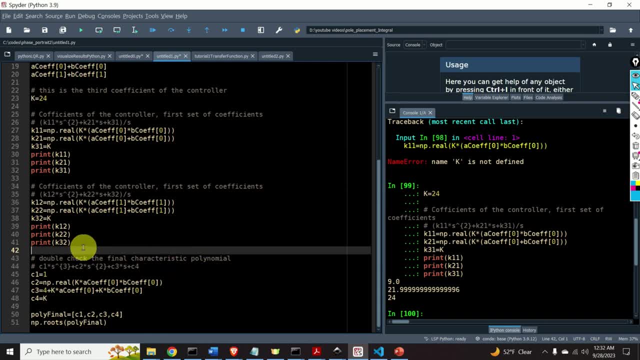 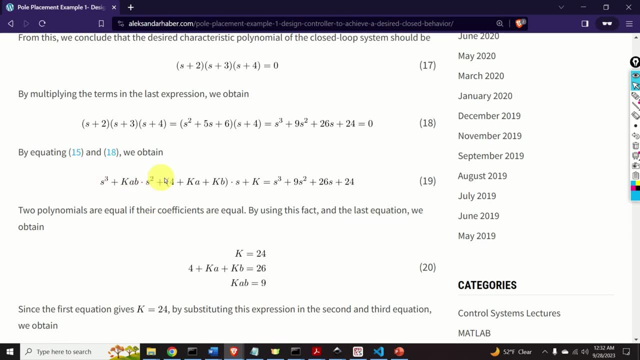 final characteristic polynomial Over here I will take the computed control parameters and I will substitute them in the characteristic polynomial given by this equation. I should obtain something like this: and the zeros of this characteristic polynomial are equal to 0. And I can substitute them in the 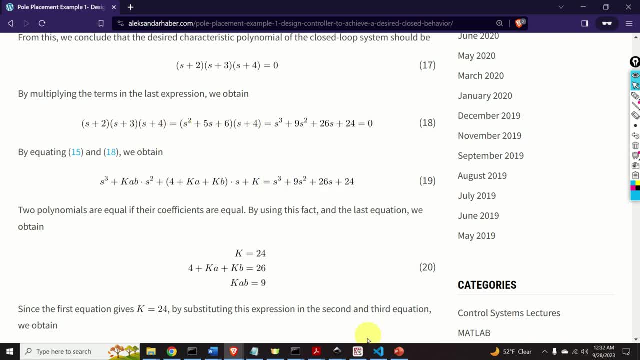 characteristic polynomial given by this equation, I should obtain something like this: and the zeros of this characteristic polynomial are equal to 0. And I can substitute them in the characteristic polynomial given by this equation, I should match the desired pole locations. Let's do that Over here. I compute the. 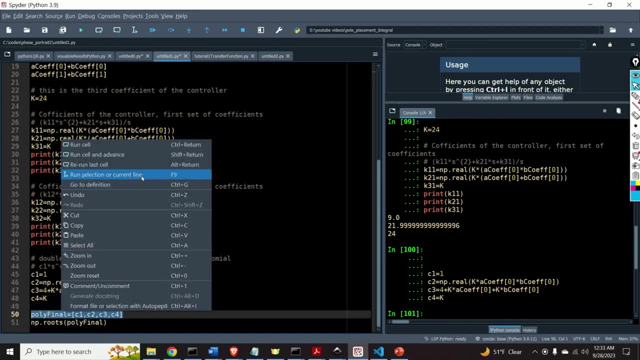 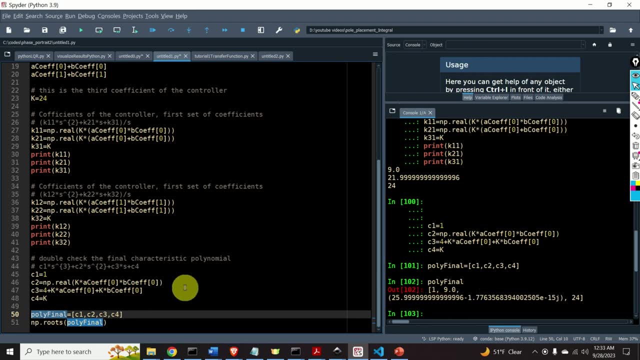 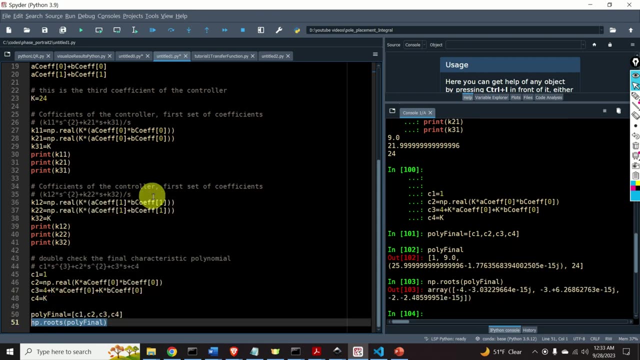 coefficients. I define my polynomial. Here it is, We can also see it- 26 and the other terms are here: 1, 9,, 26,, 24.. And let's look at the roots. Here they are. The roots are minus 4, minus 3 and minus 2.. 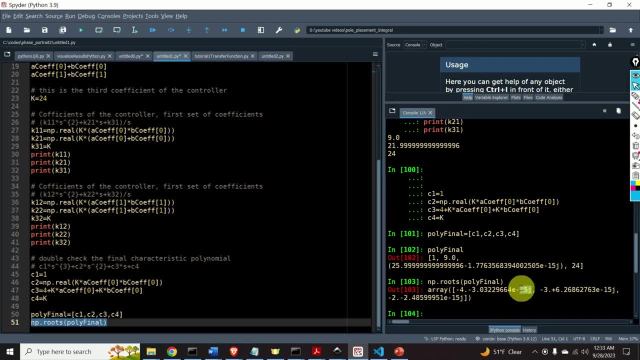 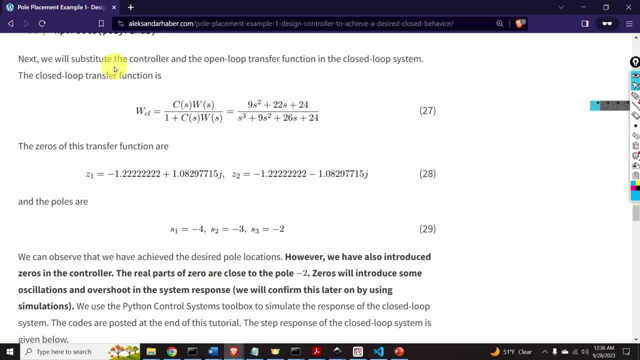 Forget about these small, complex numbers, since they are the numerical precision, And that's it. Simple as that. Next, we need to substitute the controller and the open-loop transfer function in the closed-loop transfer function And, as the result, we obtain this equation. This equation is very important. We can. 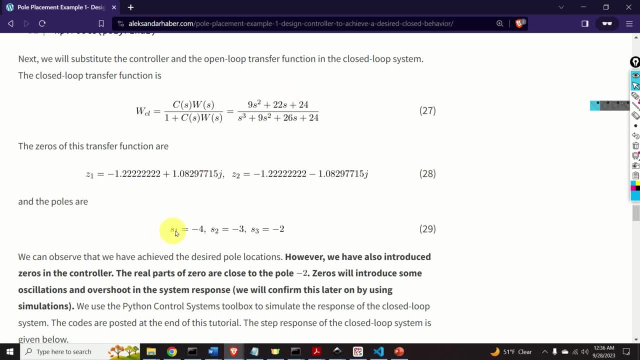 observe two things: The poles are given over here and these are the desired poles, So nothing is wrong over here. However, we can observe that we also have zeros. To remind you, zeros are zeros of this polynomial in the numerator And the zeros are given over. 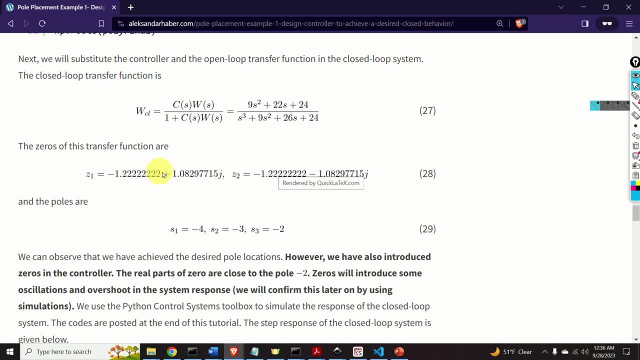 here We can see that the real part of this zero is very close to this pole. OK, To summarize, we observed that we have achieved the desired pole locations. However, we also introduced zeros in the controller. The real part of the zero is close to minus 2.. 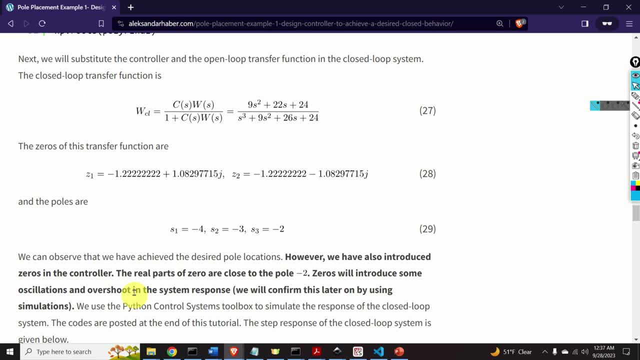 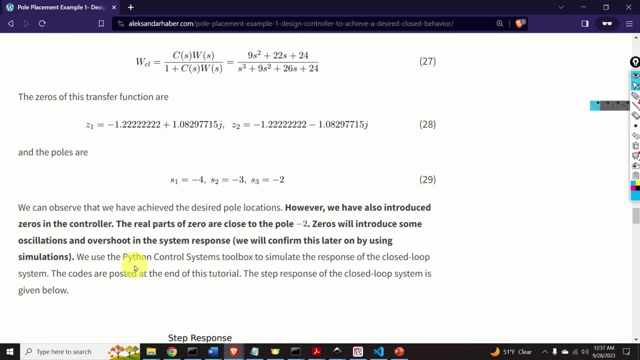 Zeros will introduce some oscillations and overshoot in the system response. We will confirm this later on by using simulations. Let's simulate the system. To simulate the system, I am using the Python Control Systems Toolbox. This is a very powerful control systems toolbox. It's completely free. 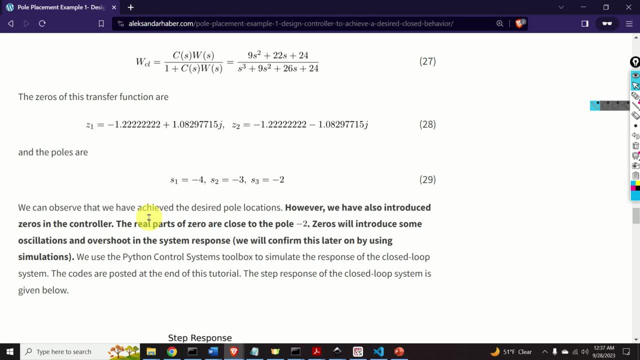 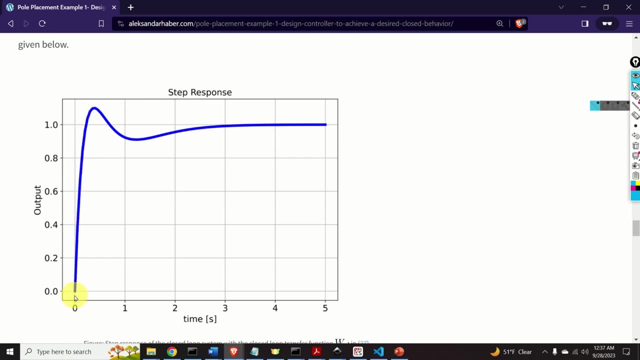 And I made several tutorials on how to use this toolbox. Links to my tutorials are given in the description below. First, let's compute the step response of this system. The step response is given over here. We can observe two important things from this step response. First, 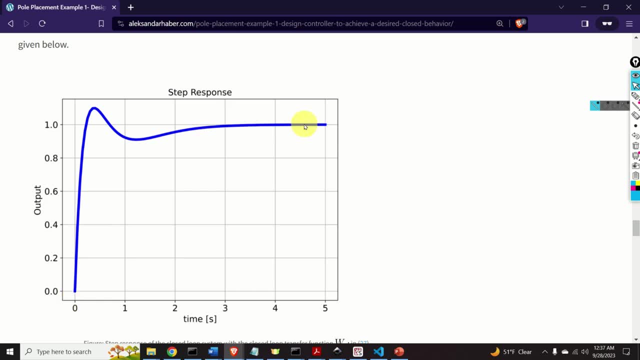 of all, the steady state error approaches zero. This is because the input signal is one and in steady state our system tracks one. One is 0,. two is zero. In this case, the steady state error approaches one. So we can compute the step response of this system. 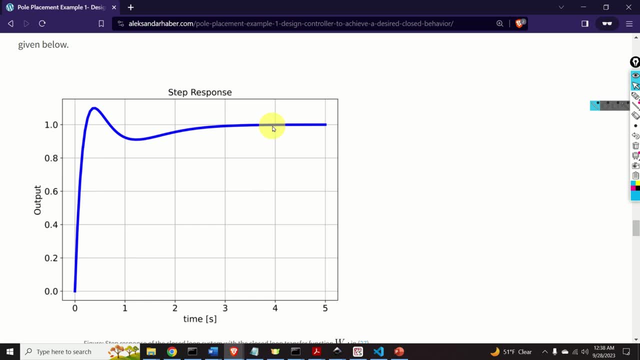 This is because the input signal is one and, in steady state, our system tracks one, So perfect. however, we can see this phenomenon over here, that is, we can see an overshoot and, as i will show it in one second, this overshoot is a direct consequence of introduced zeros in our control. 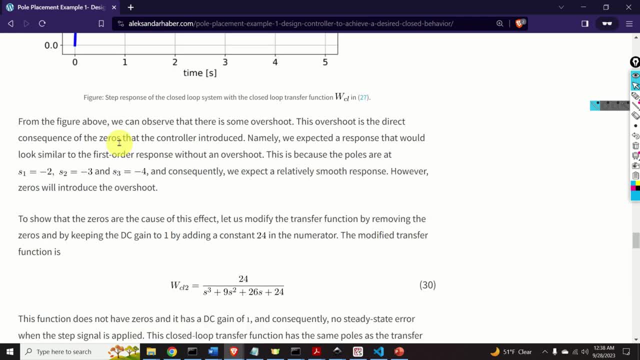 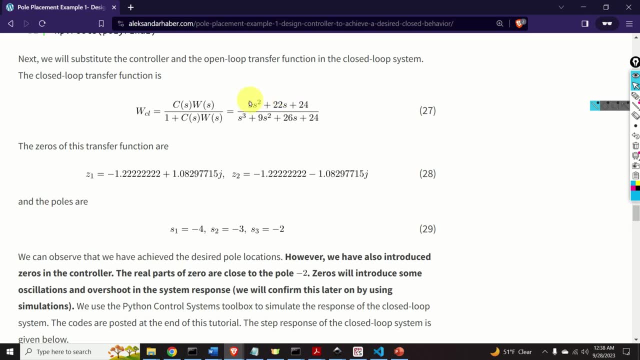 system to see that let us modify our transfer function. here is our original transfer function and let's eliminate zeros from our transfer function. we do that by simply dividing this transfer function by this term over here, and we multiply the result by 24 to obtain this expression. 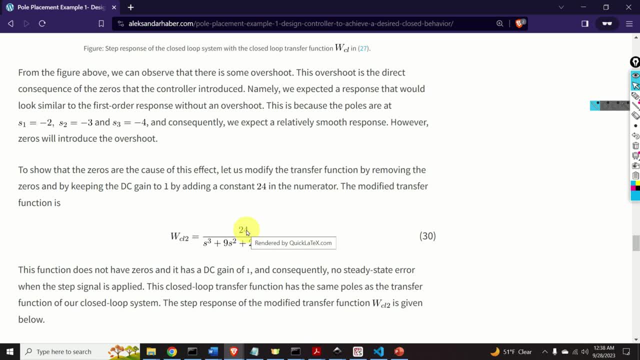 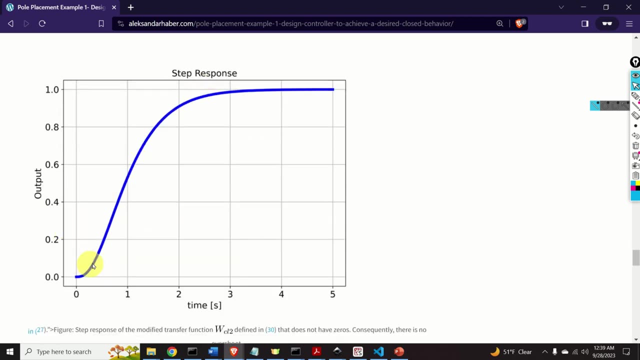 why introduce here 24? well, i introduced 24 since i want to make sure that my steady state dc gain is equal to 1 and let's compute the step response of this system. here is the step response. we can clearly see a very nice and smooth step response. this is because we don't have zeros over. 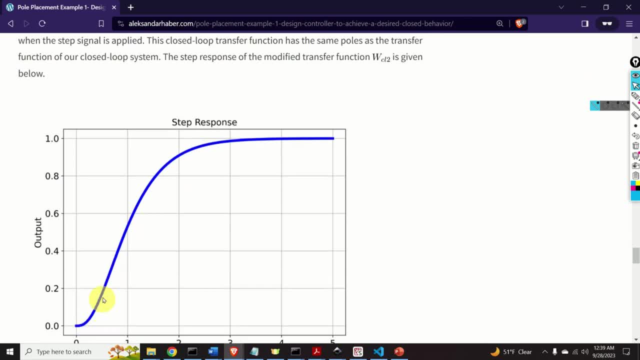 here and this system exactly behaves according to what we want. that is, we want poles to dominate the system. response: that is, we should see the terms in our step response having this form: plus minus minus 2t, plus minus e to minus 3t and plus minus e to minus 4t. that is, we should see something that looks like: 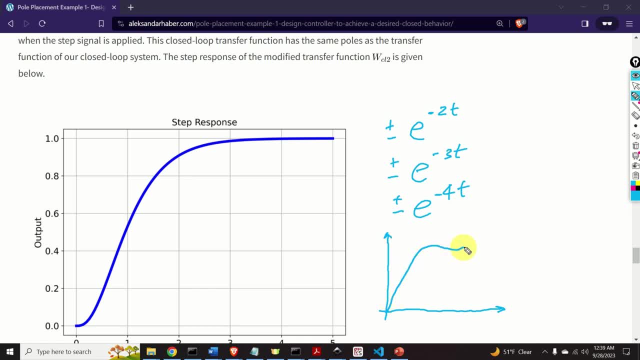 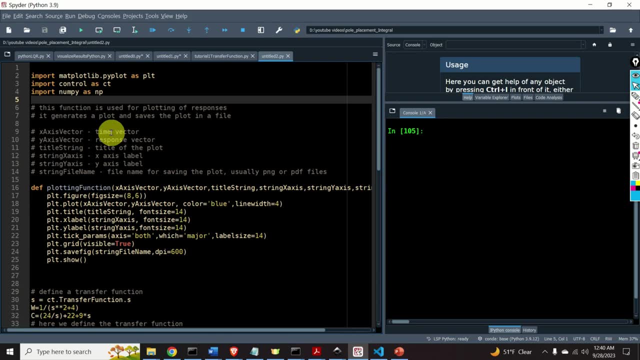 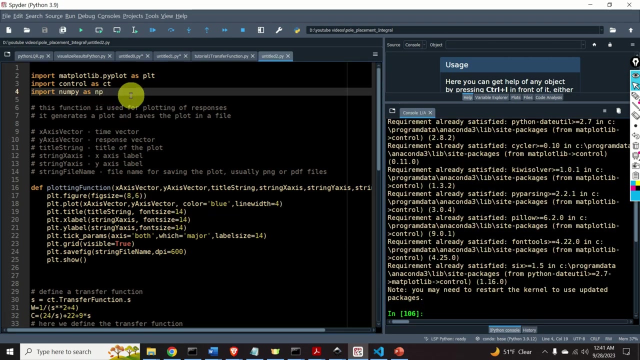 the response of the first order system. next i will explain the python code that i use to simulate the closed loop response. i'm using the control systems toolbox. to install the control system toolbox you will need to type in your command prompt: pimp, install control and this will install the control systems toolbox. okay, first i need to import the necessary 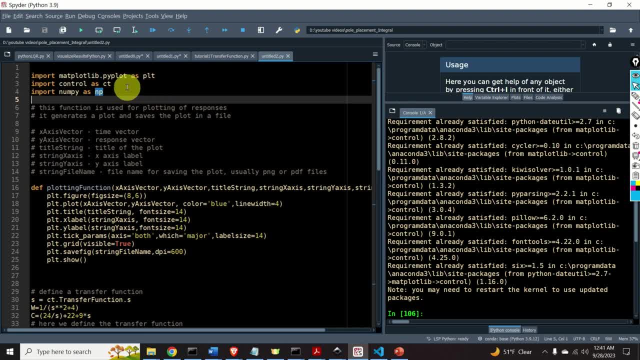 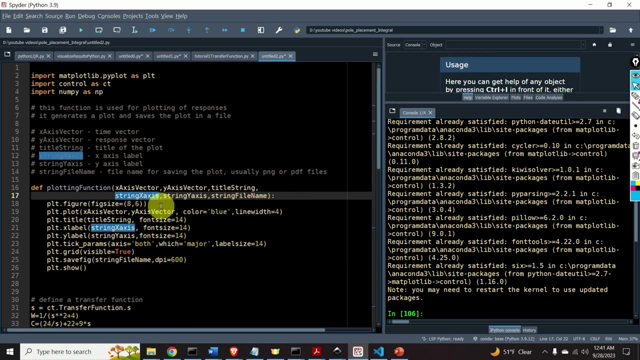 libraries. i need the plotting library, i need the control system toolbox- and note over here that the control system toolbox is imported as ct- and i need numpy. over here i wrote a simple function that is used to plot results. This function accepts several arguments. It accepts the time axis vector. 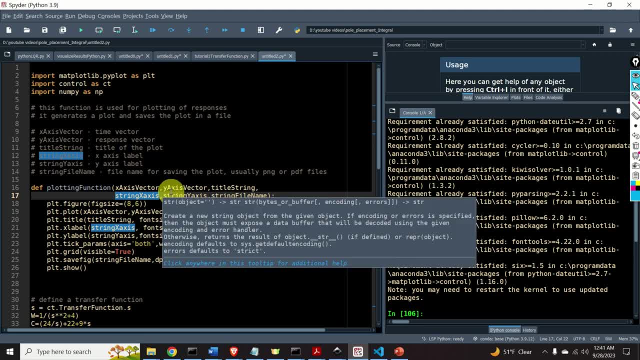 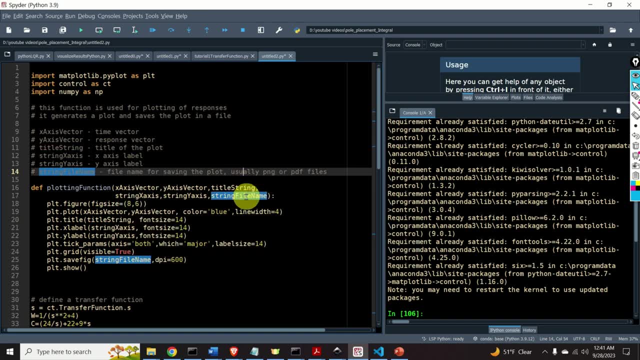 the y axis vector, the title of our plot, the x label, the y label and the string file name. This input is used to give the name to the saved file. This function will plot the graph and it will save the graph in this file. That is, the name of the file is specified. 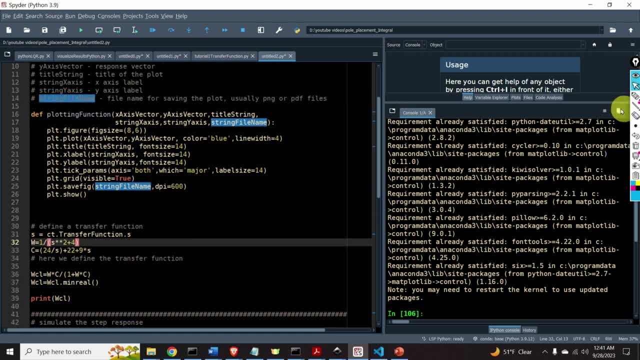 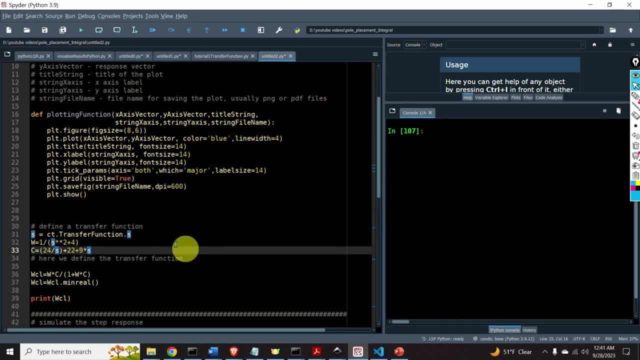 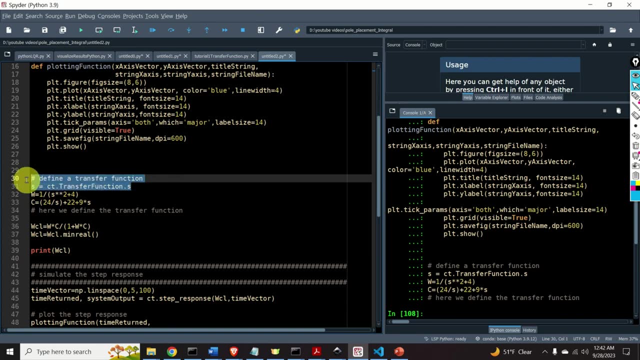 by the user. Okay, so let's define our transfer function First. let's erase this part and let's clear this part. Here's how we do that. We simply specify s to be a complex variable. We call ct. this is our control system's library object. and we call ct. this is our control. 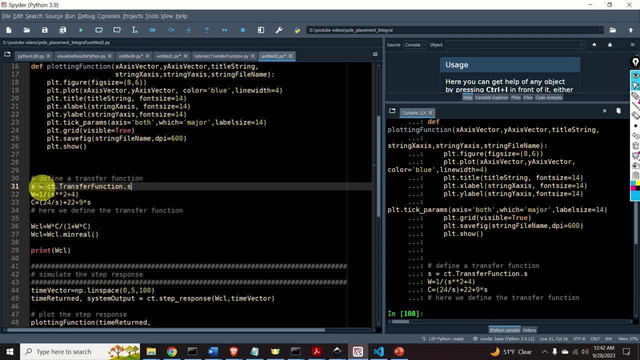 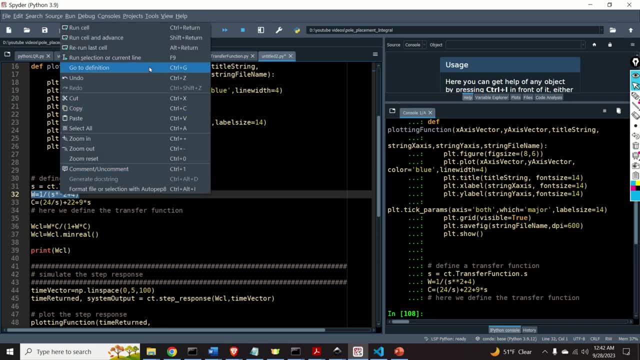 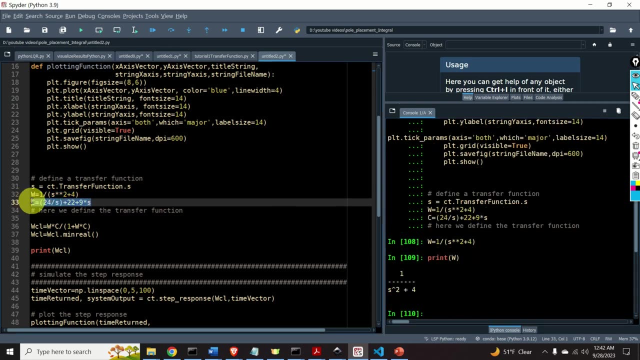 system's library object and we call ct. this is our control system's library object and we say transfer function. dot s is equal to s, And here it is. We can simply define our transfer function. here it is. To show it, you need to type print w, And here's our controller. 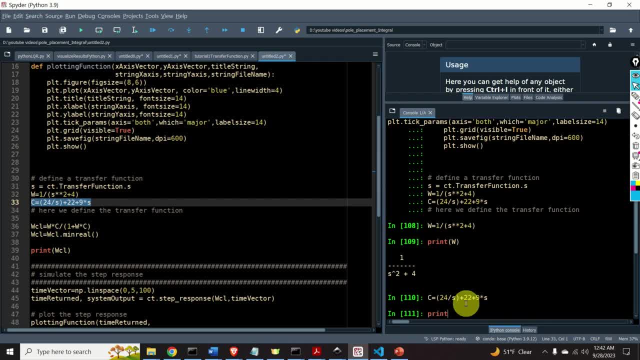 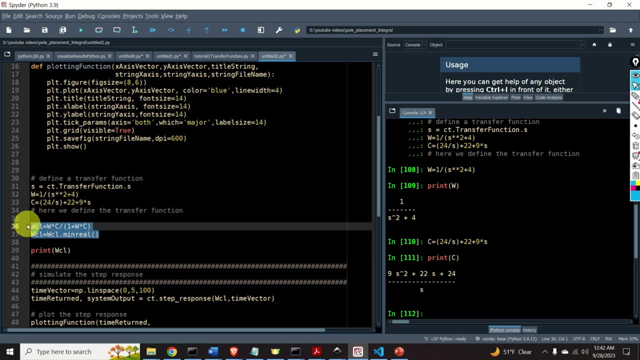 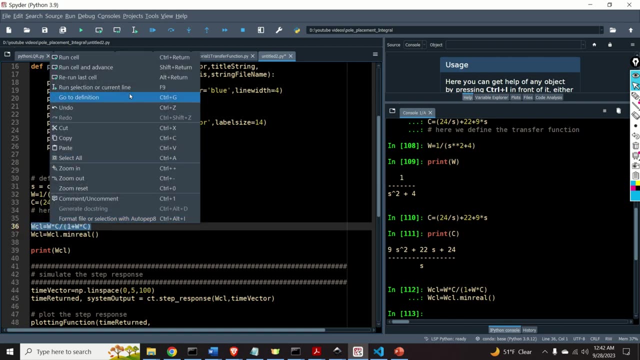 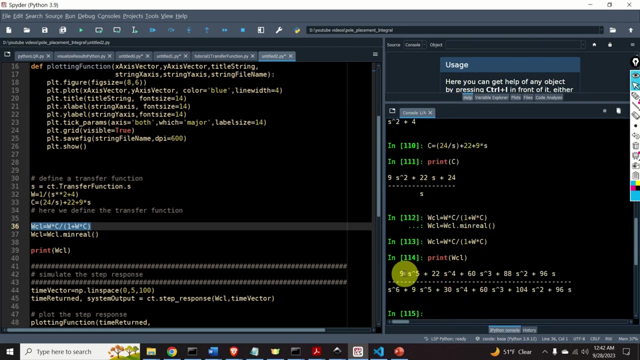 Let's print our controller. Here it is. Next, let's define the close loop transfer function. Here it is and know what I'm doing over here. First I will execute this part to show you. If you type print vclosed, look what you will get. Hmm, very complex expression. Let's go back to the tutorial and 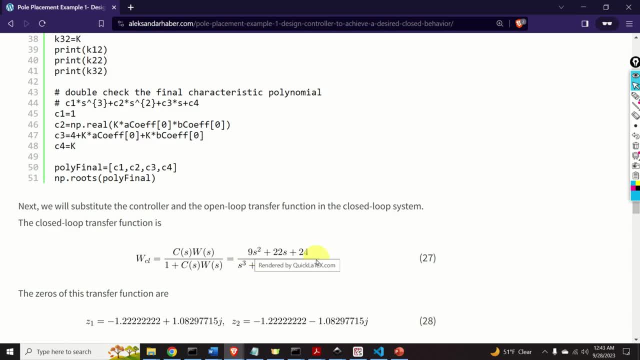 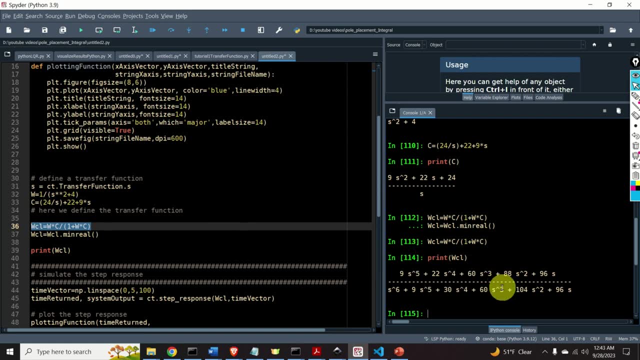 let's see our transfer function. Aha, the transfer function should look like this. However, we obtain something like this: Well, you need to cancel some zeros and pulls over here, And to do that, you need to call this method mean real And, consequently, that's why I'm defining the transfer function like: 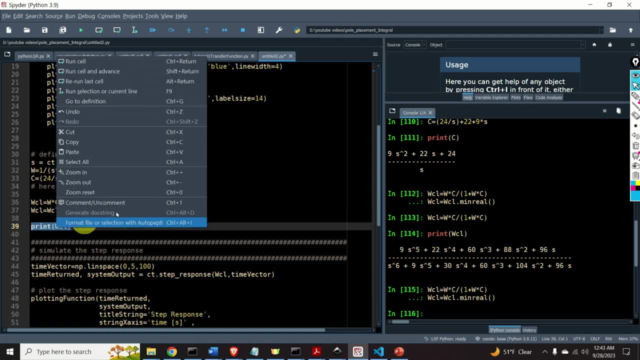 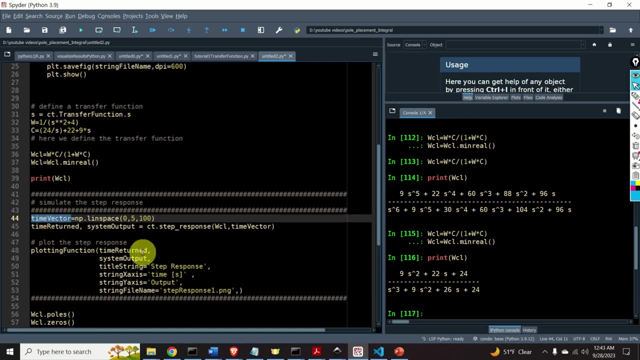 this, And once I do that, let me print the closed loop system Here. it is Perfect. And let's simulate the step response. First of all, we need to specify the time vector 0 until 5, with 100 steps. 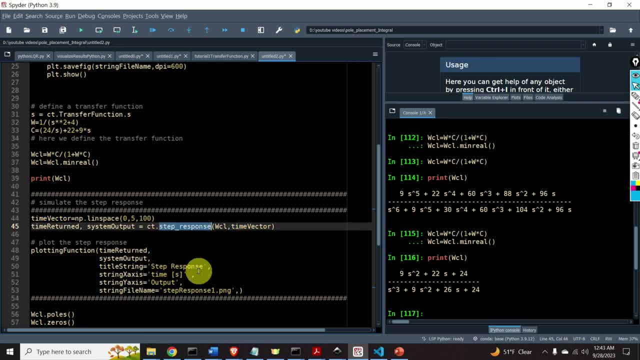 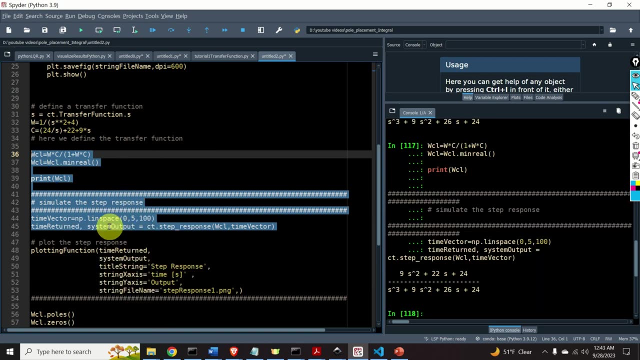 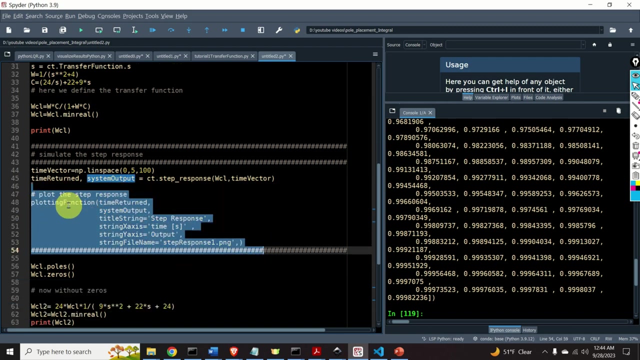 And over here. I'm calling the step response function. I specify the name of the transfer function, the time vector, and, as the result, I will obtain the time and I will obtain the output. Let's see the output Here it is, And let's plot the step response. I'm calling the function that. 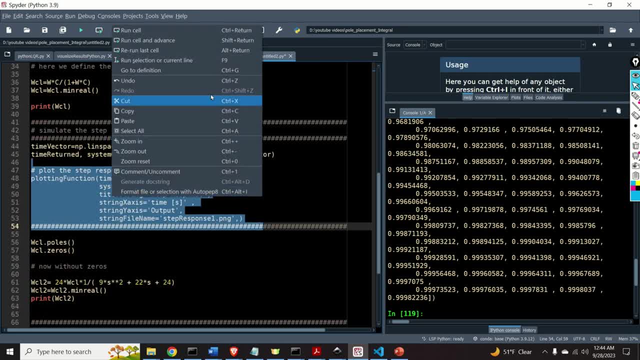 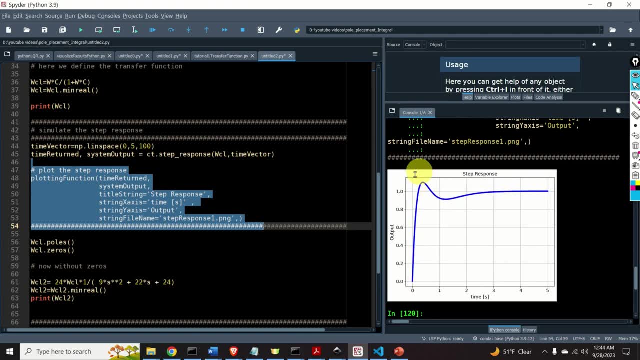 I defined at the beginning of this video tutorial. Here it is, And voila, here's our step response. Again, we can see an overshoot, and this is the phenomenon that we don't like. However, we have to live for the time being with this overshoot. Let's compute the poles and 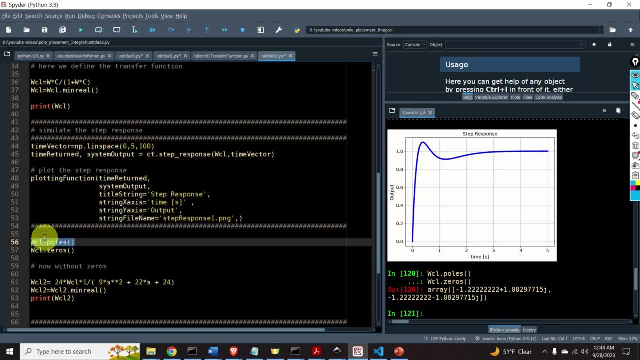 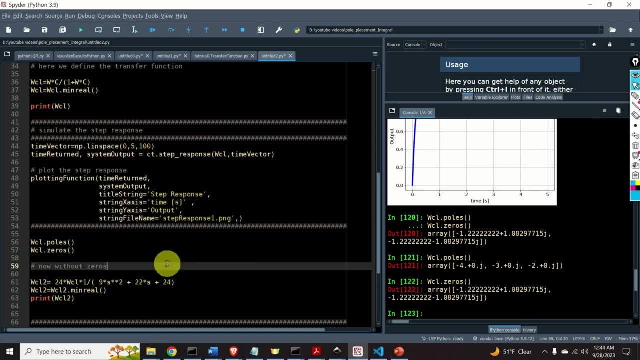 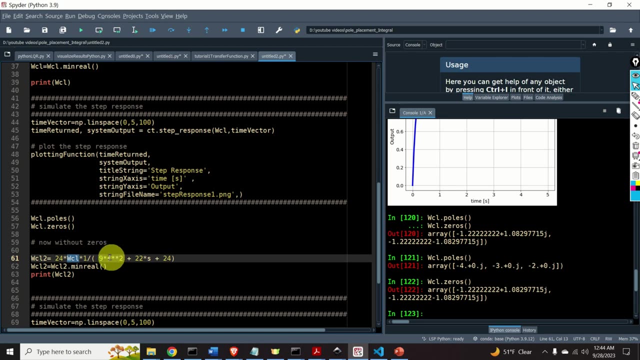 zeros of our transfer function. Here are the poles and here are the zeros. Perfect, Now let's define a new transfer function. Let's say we have a function without zeros. To do that, we simply divide our closed loop transfer function by this.